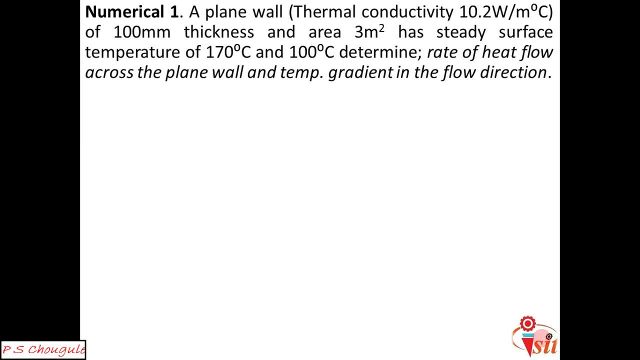 Watt per meter degree Celsius of 100 millimeter thickness and area 3 meter square has a steady surface temperature of 170 degree Celsius, and 100 degree Celsius Determine heat flow across the plane wall and temperature gradient in the flow direction. So let us drag out what they told you. Here it is a plane wall. One surface is at 170. 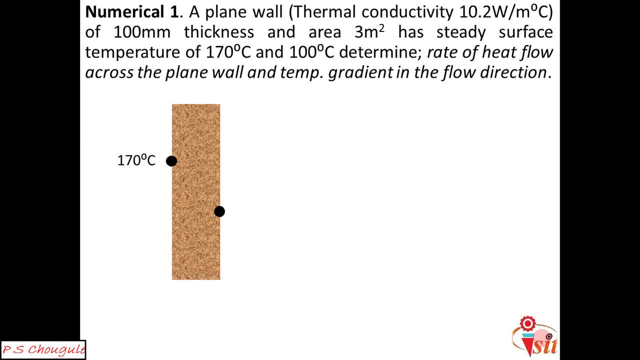 degree Celsius, Another one which is at 100 degree Celsius. That means heat will flow from 170 degree Celsius to 100 degree Celsius. Now, by this means we will get the direction of heat from 170 degree Celsius to 100 degree. 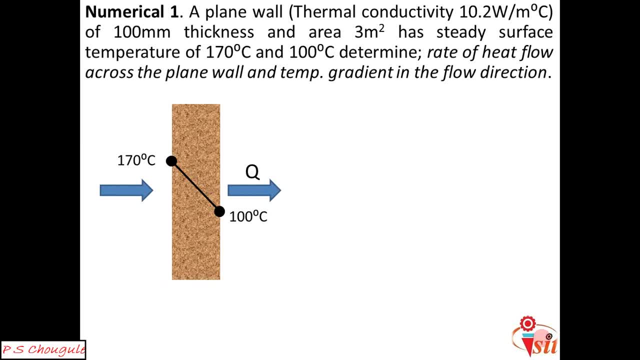 Celsius. Let us say the heat flow rate is of Q. Now the area of the plane wall is of 3 meter square And the thickness of wall is of 3 meter square. Now, remember that since we are working in SI unit, so we need to convert that millimeter. 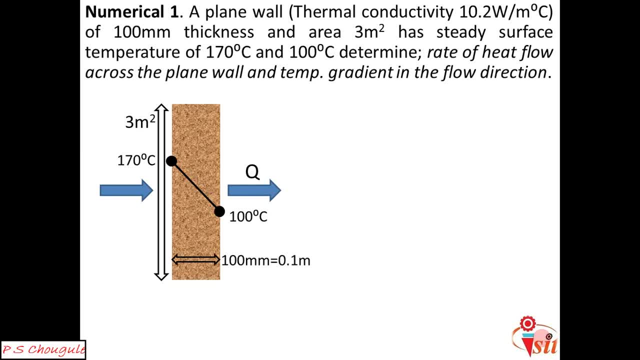 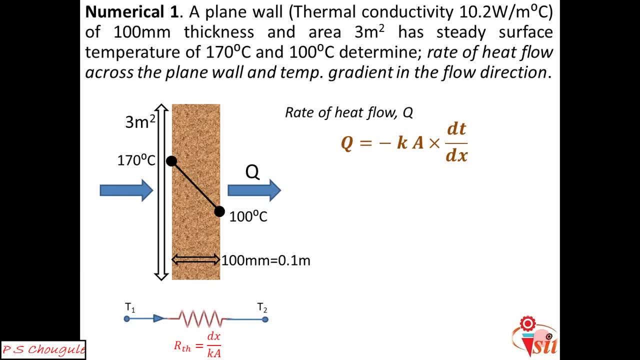 dt is the temperature difference we have to take here, final minus initial, and dx is the thickness of that slab. So here q is equal to: if I put the values, respective values of that quantities, I will get the value q. Remember that you have to write here negative sign to compensate this difference temperature. 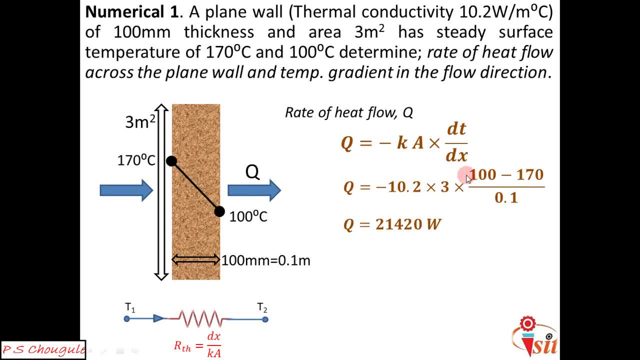 difference, because always here the lower temperature minus higher temperature, Heat flows from 170 to 100 and we are taking here difference 100 minus 170.. So the answer is in bad. So you may write it in this way: 21.42 kilowatt. 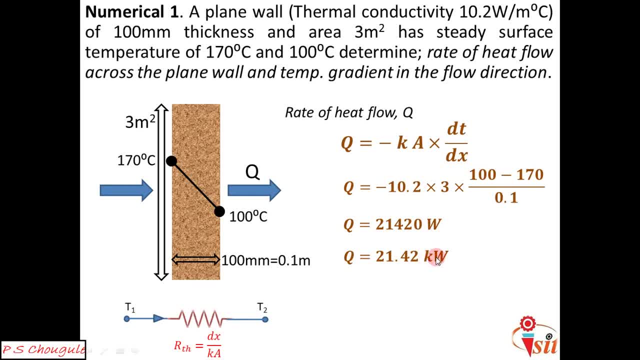 This is the first part: to find out the heat flow across the plane wall. Now, secondly, they told you to find the temperature gradient. So for that you can write temperature gradient: according to Fourier's law, q is equal to minus ka into dt upon dx. 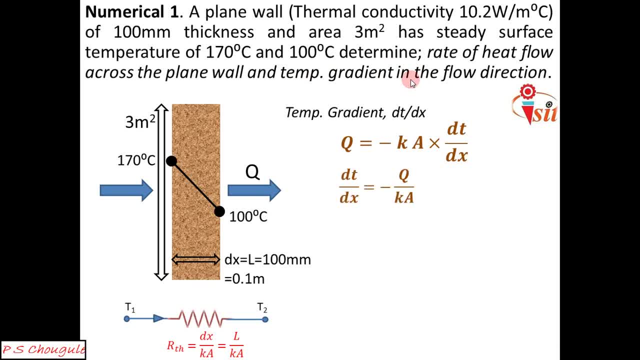 You can take dt upon dx, Okay, On the one side. So you will get one formula which is minus q upon ka. Since we have derived the value of q, you have to write here: value of q in watt only divided by k into a. 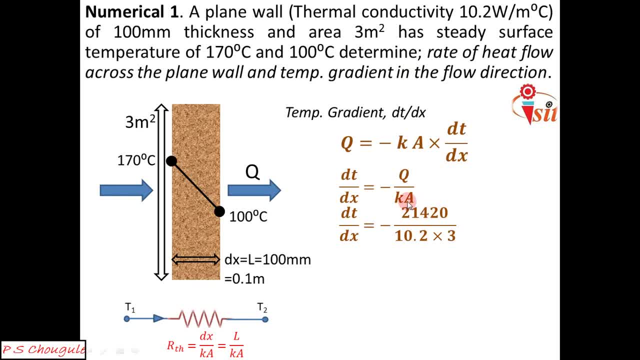 K is the thermal conductivity, a is the area, So that you will get this answer, which is in degree Celsius per minute, Sir. Okay, Now we have calculated this by using the value of q, which we have formed, or we have calculated In another way. you can find out the value, that is, temperature gradient, in this way also. 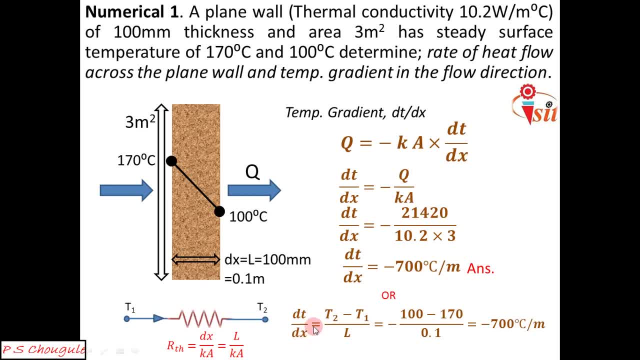 dt upon dx, which is the temperature gradient, which is equal to. T2, means the last temperature minus final temperature, Initial temperature. T1 divided by L. L is the length, 100 minus 170 divided by 0.1, which is equal to again the same minus 700 degree Celsius per meter. 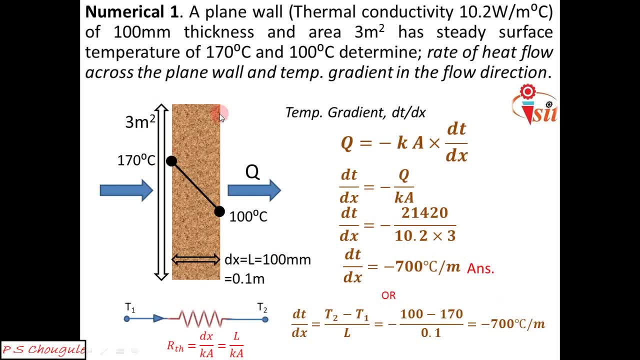 You can write this. instead of drawing all this diagram, You can write it in a electrical analogy way. Okay, In this way, T1 is the temperature 170 degree. T2 is the temperature 100 degree Celsius. This one, instead of this wall, I have write it over here. 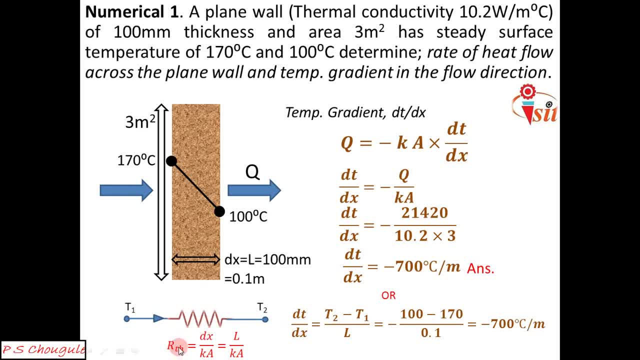 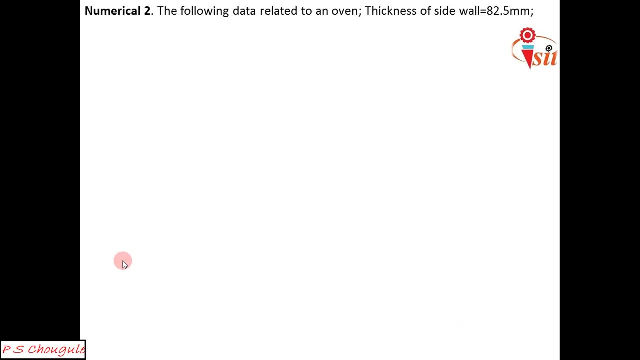 One resistance, which is the thermal resistance, is equal to dx upon ka. Let us take one more example. Okay, Okay, Let us calculate this by using the value of q, which is in degree Celsius per minute. Let us write this further: T2 is the thermal resistance, k? ie. t2 is equal to k? ie write this. 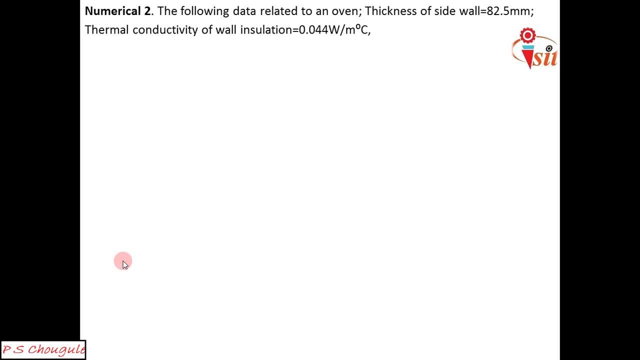 T2 is equal to k. ie, l, i. Let us write this. Let us write this: where, where is z? Where is z? If it is z, then why is it z? z is equal to c. Yeah, let me write this. 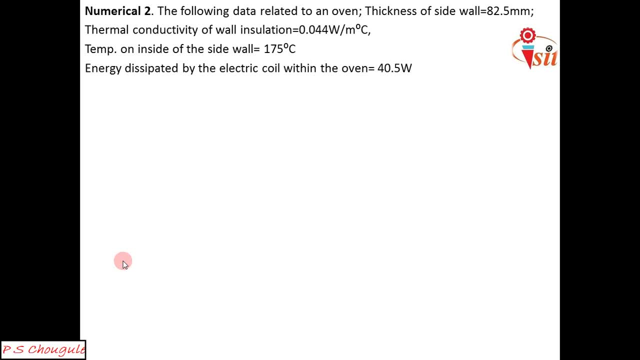 So this is the thermal resistance k ie- current density. k ie- current density d. Yeah, the area of wall surface, so that the temperature on the other side of wall does not exceed 75 degree Celsius. So let us draw the diagram which we have drawn previously. 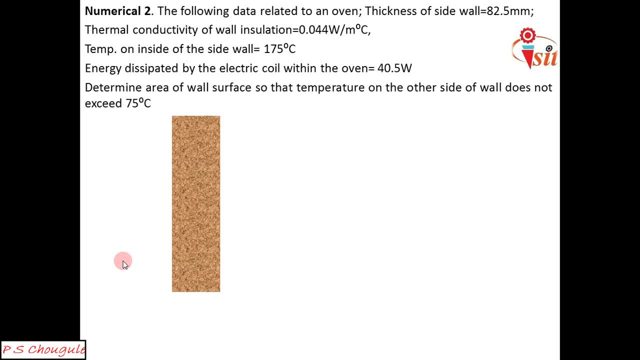 Here it is the thickness or the side wall of that oven. The inside temperature is of 175 degree Celsius and outside temperature is of 75 degree Celsius. So heat will flow from 175 degree Celsius to 75. That means the heat flow direction is in this way and they have given the energy dissipated. 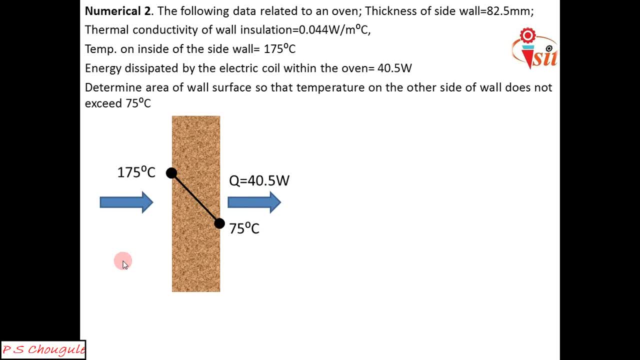 by the electric coil, which is 40.5 watt. Now this is the surface area which we need to find out. They have given the thickness, which is in mm. We need to convert that into meter, 82.5 mm, which is nothing but 0.0825 meter.